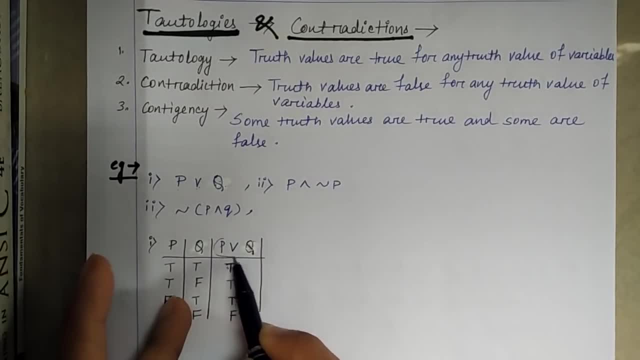 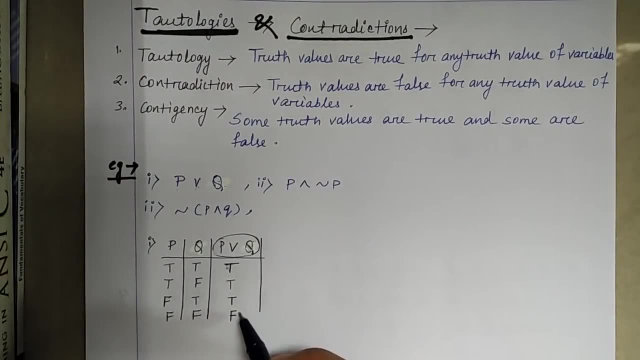 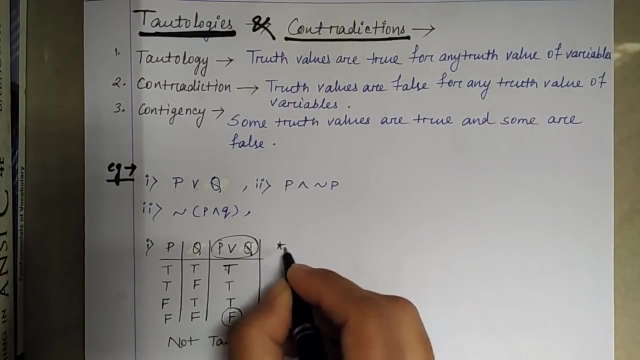 so if you are getting this part, this last column, value, all are true, then only it will be called as tautology. but are you getting it true for all? no, right, because for this one it is false, so this is not a tautology. then let's say, i'll take another example: p or negation p. 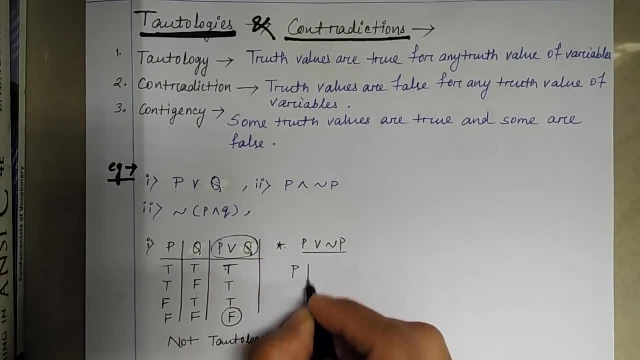 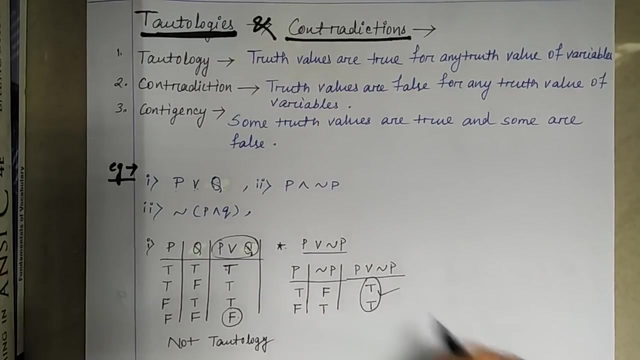 okay. so p and negation p- only two column you'll be having, so that you know for true it is false and for false it is true. so when you perform p or negation p in, or if either of the truth value is true, then you'll be getting the value as true here. so in the last column we have got both the values as. 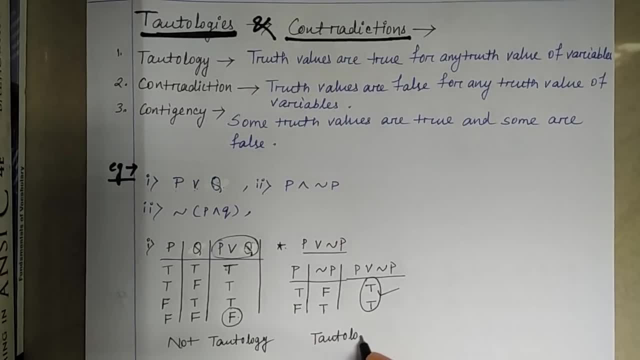 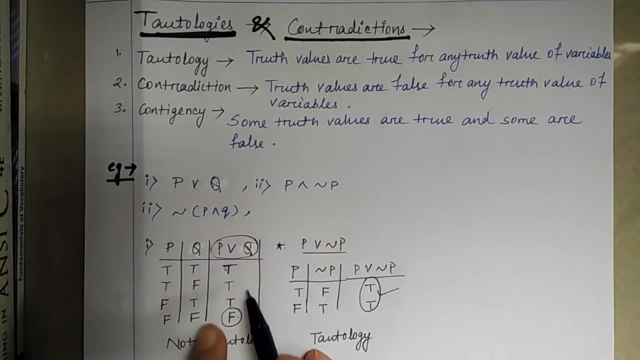 true. so this is known as tautology clear. then the next one is control, control, contradiction. what is contradiction when all the truth values are false of any value of the variable? so likewise you can see the first example: p and q, two variable. and in the last column, if you 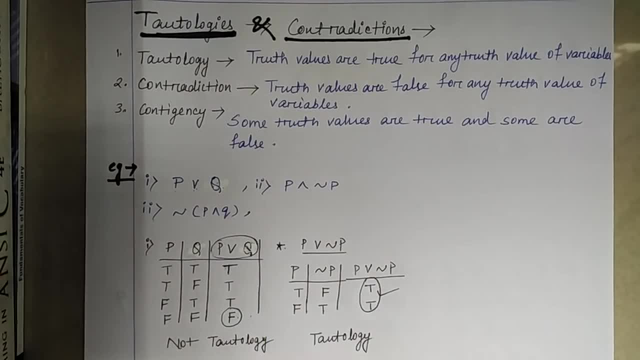 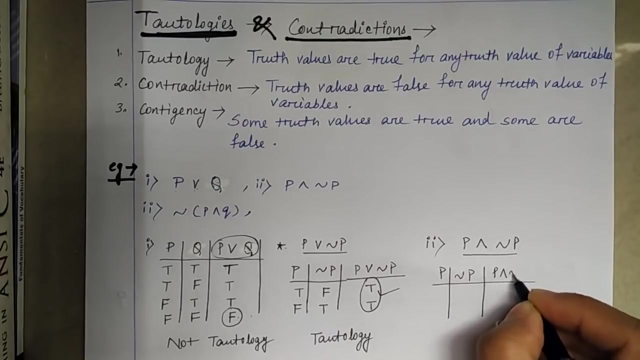 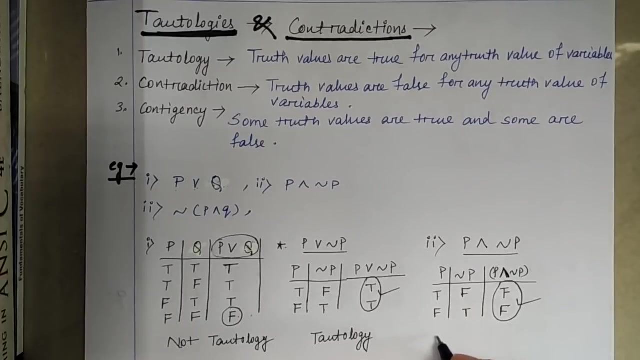 would have got all the truth values as false, then it would have called as contradiction. we'll see the second example, that is p and negation p. so we'll obtain two column, first p and negation p, and last one is p and negation p at a time. so this will be true, false and false true, right in end operation. both the values are true. then only you'll be getting the truth values are true, but here one is true, another is false, so this is false. one is true, another is false, so this is false. so what you are getting in the last column? both the values are false, so this kind of table is called as contradiction. 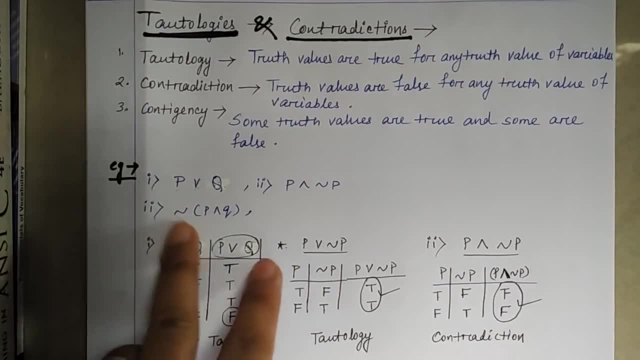 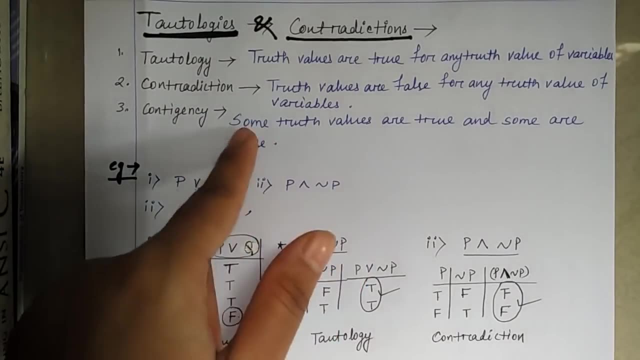 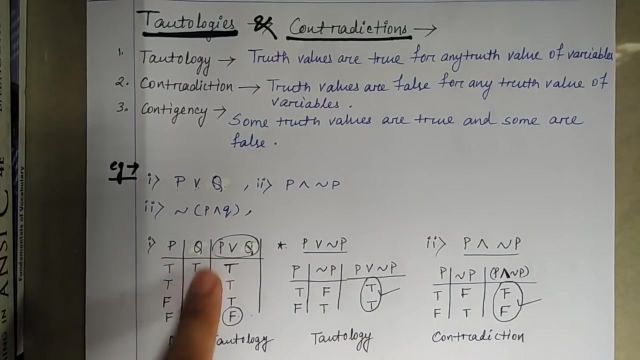 now, uh, the third example is negation of p and q, and third definition is contingency. contingency is if some of the truth values are true and some are false. that is called as contingency. in the first one we have seen that three are true and one is false. so it is. it is mixed up true and false, so we can call this as contingency. if it is asking whether it is tautology or not, you should say it is. 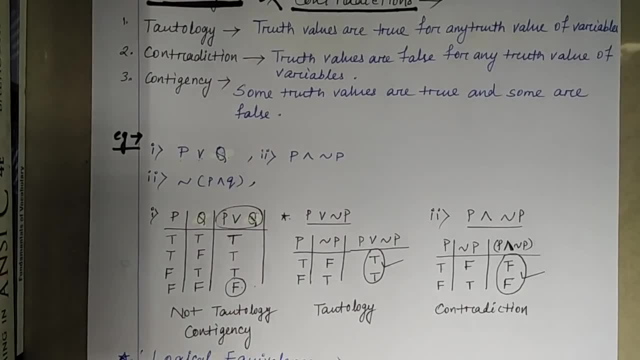 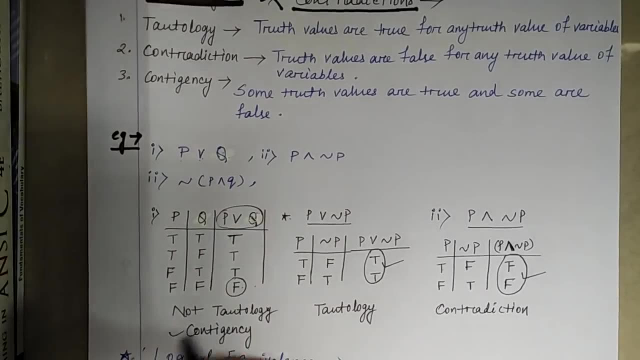 not tautology. if it is asking contradiction or not, you should say it is not a contradiction. but if it is asking whether it is contingency, you should say contingency, yes, it is a contingency. why? because three values are true and one value is false. so it is mixed up, true and false, and 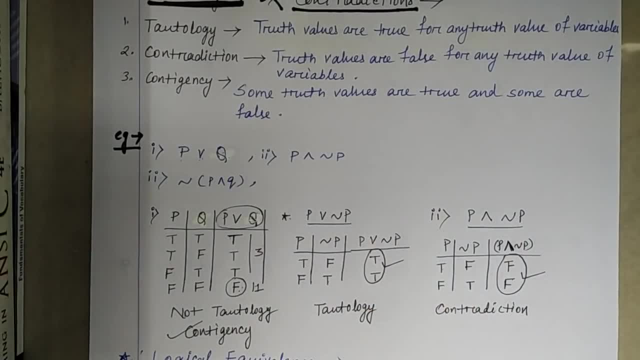 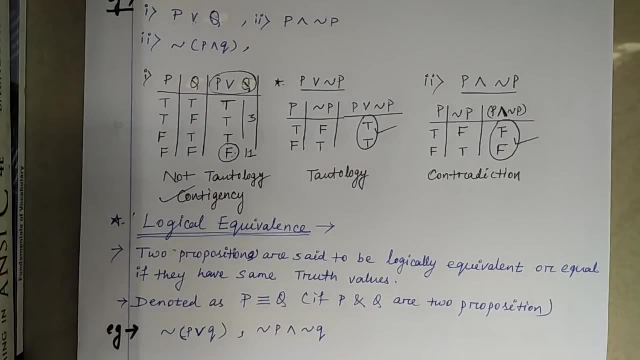 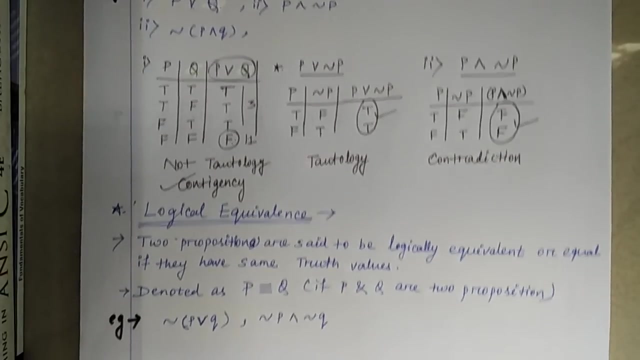 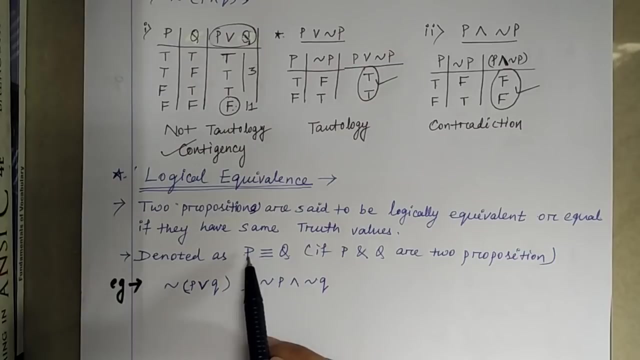 according to the definition, it is a contingency. then we'll see the logical equivalence. actually, few more important points are there to be covered that some of them are logical equivalence, then conditional by conditional statement. so what is logical equivalence? according to logical equivalence, if you have taken two propositions, let's say p and q, they will be called as logically. 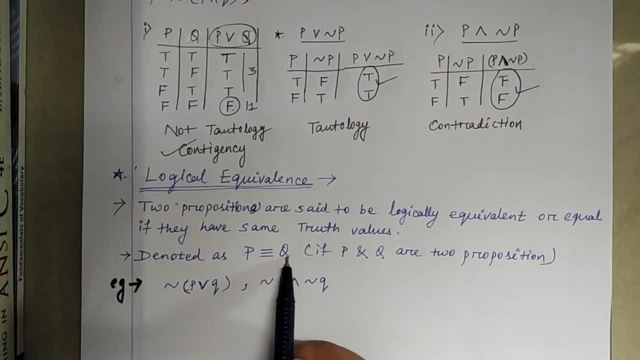 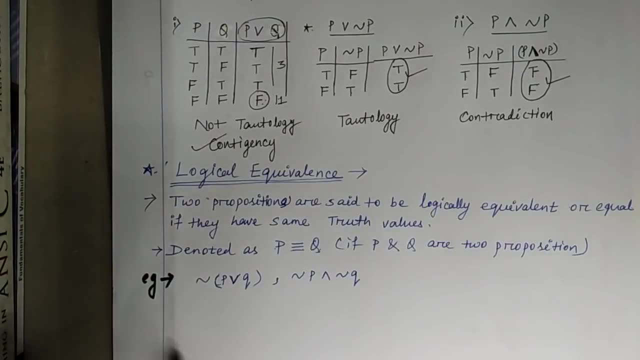 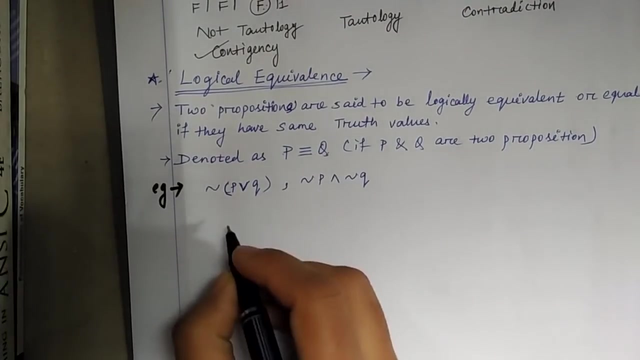 equivalent or equal if they maintain the same truth, value or same truth table in the last column. okay, so we'll see two example here, negation p and q, and negation p or negation q. so for example, first one will go for. so how can you write that? 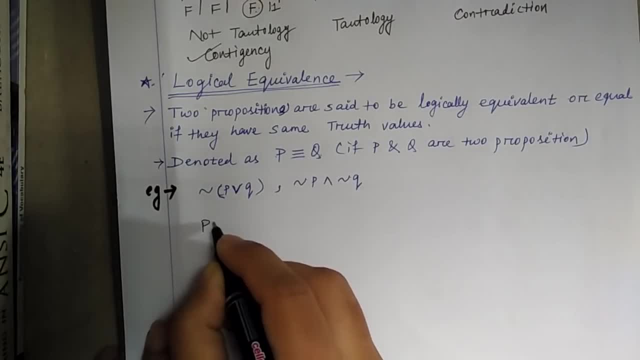 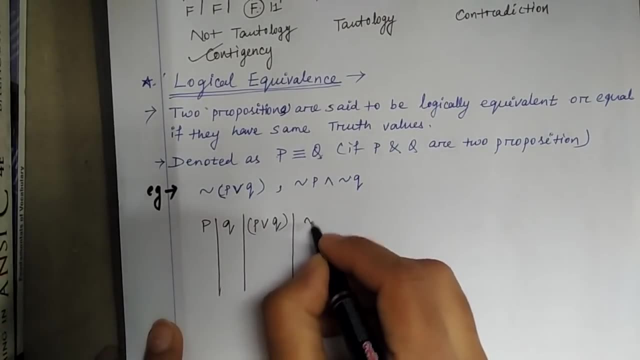 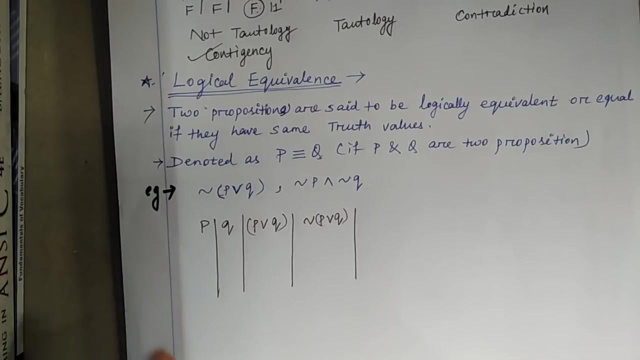 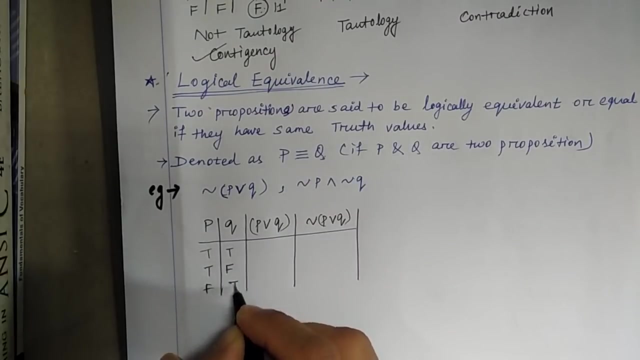 how many columns will be there? p q, p q together and p q the original one. okay, so this is a or symbol. we'll try to maintain the truth table. so in the or one, what you get all true and last is false. if you take the negation of that, what? 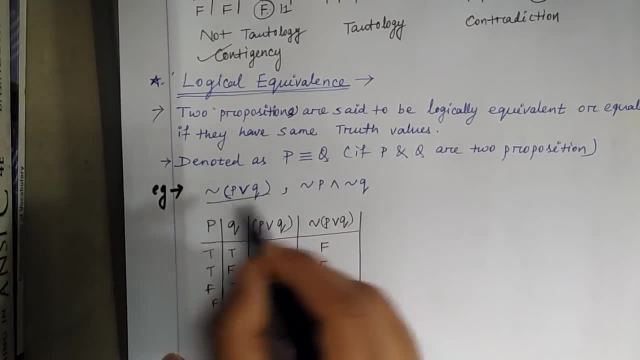 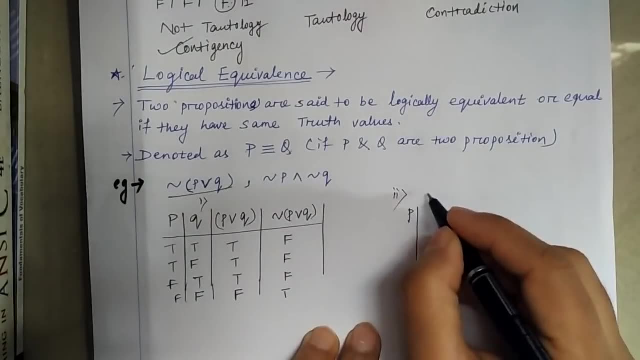 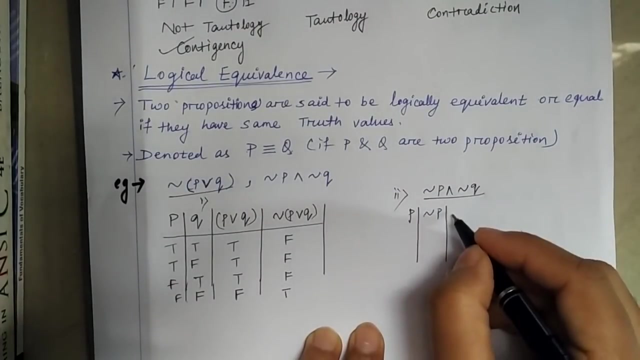 you will get all false and last is true. so this is done for the first one. now we'll see for the second one. so first is p, because it is has asked for negation p and negation q. first you'll be writing p, negation p, then q, negation q, then you have to perform and opposite of that, you have to. 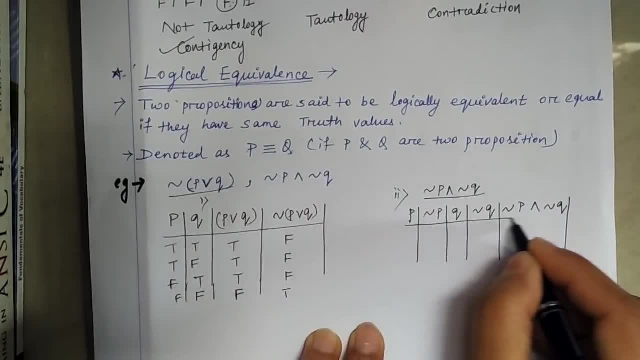 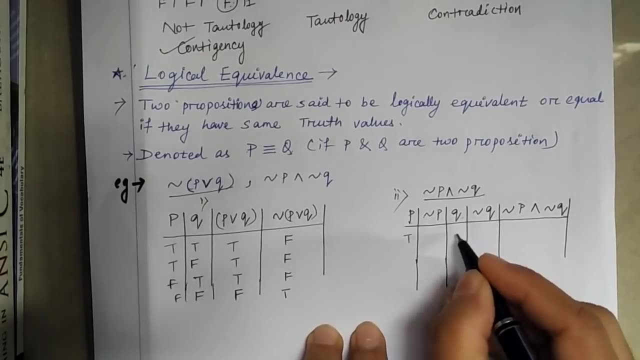 write the operation of negation p and negation q. so always try to write in a systematic manner. so when you have two variable, it will be true, true, true, false, false, true and false, false. and what will be negation p, opposite of it? so false, false, true, true. 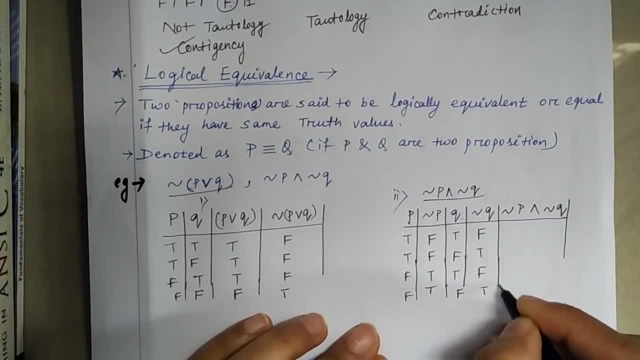 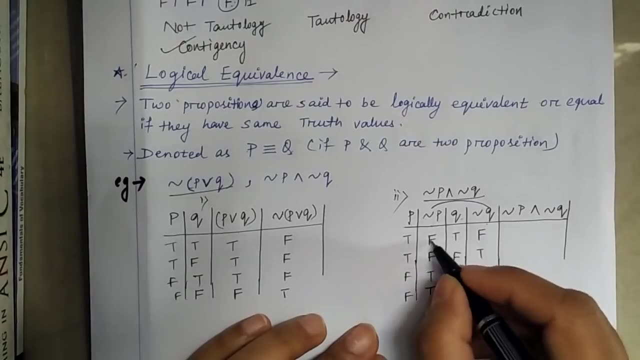 and here false, true, false, true. so when you perform operation and in between the two you will get a, this two, and means both should be true, otherwise it will be false. so first one you are getting is false, second you are getting is false, third is also false and now last one is true. so when you 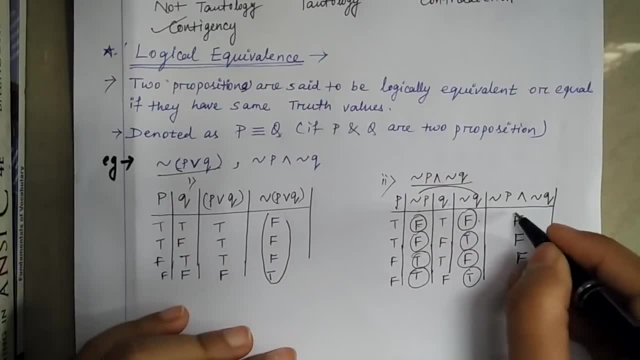 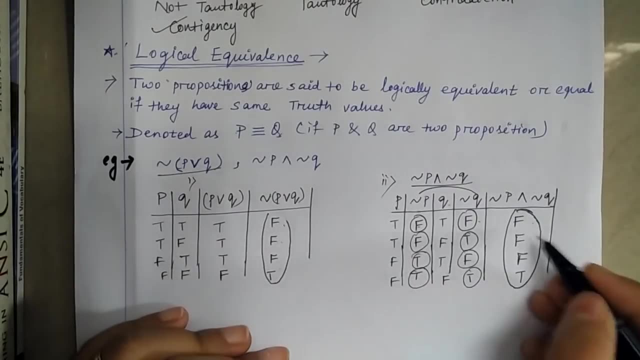 see the last column of the first statement or first expression and last column of the second expression. it is exactly same right: three false, one true. three false, one true. so, according to the definition, when you write the first one, you will get the negation p and negation q. 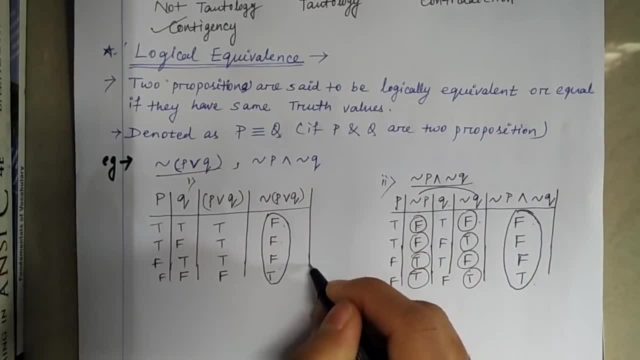 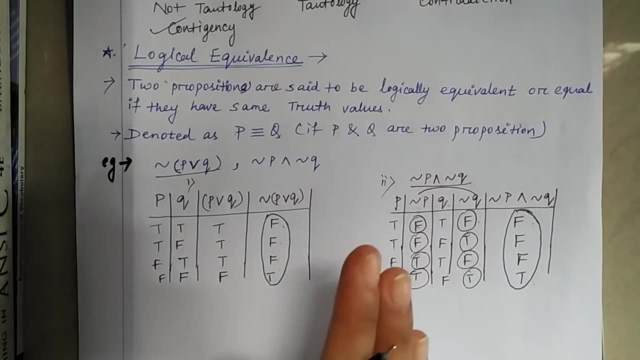 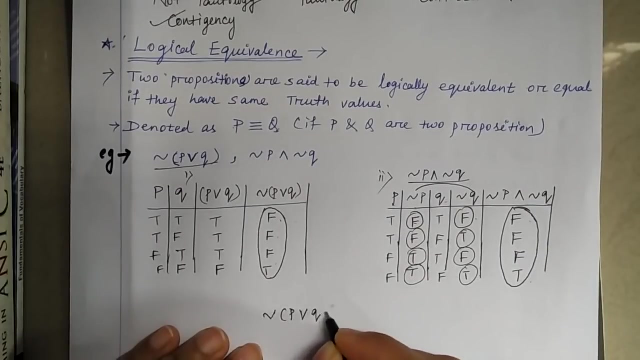 obtained the given expression and in both the expression, if the last column obtained is exactly same or if the truth values in the last column is exactly same, they are called as logically equivalent. so here we can write it as: negation of p or q is equivalent to negation of p and 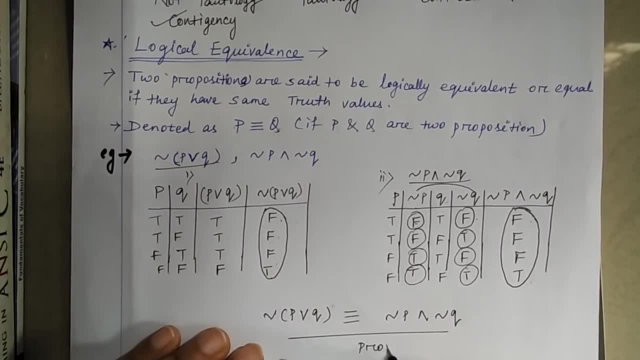 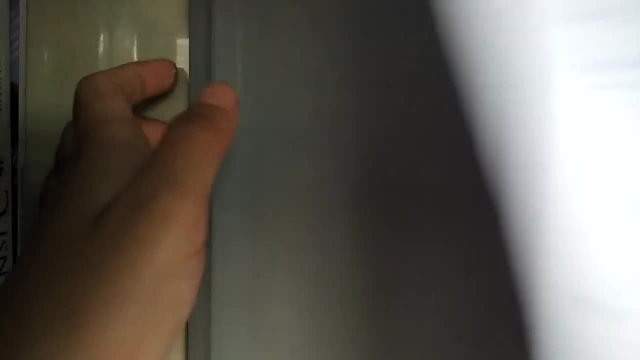 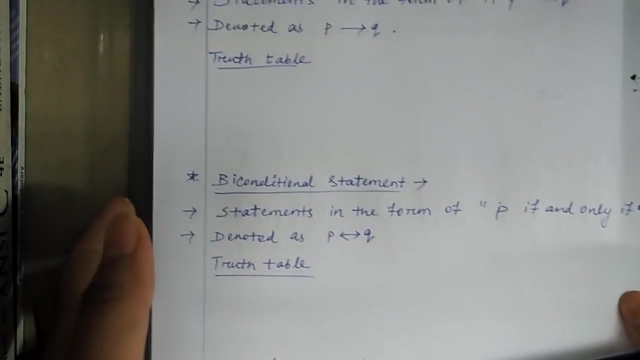 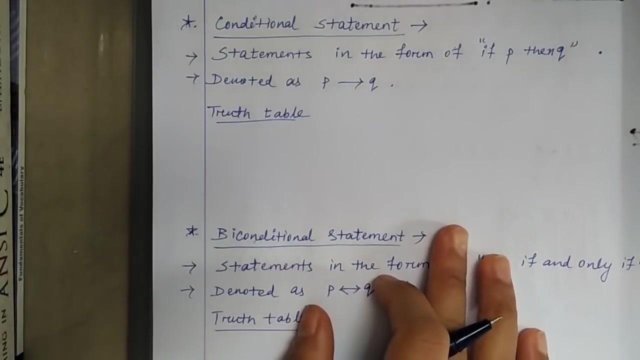 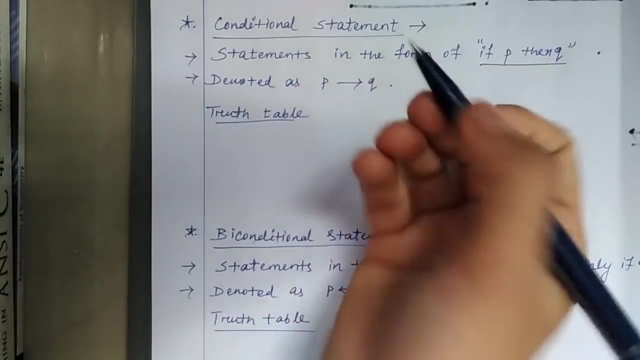 negation of q. so this is proved you clear. now we'll see some conditional and by conditional statement. so first is conditional statement. conditional statement is whenever in the statement you find the form if p, then q, that is called as conditional statement and it is denoted as p tend to q. so we'll 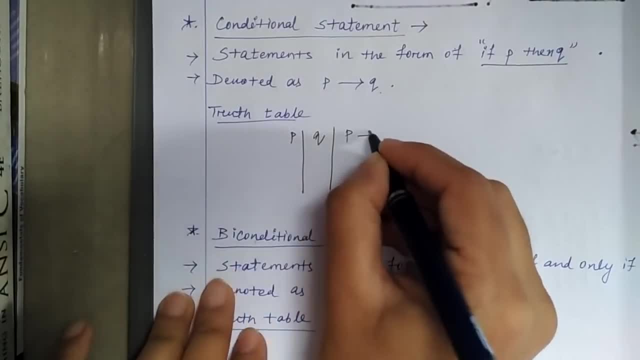 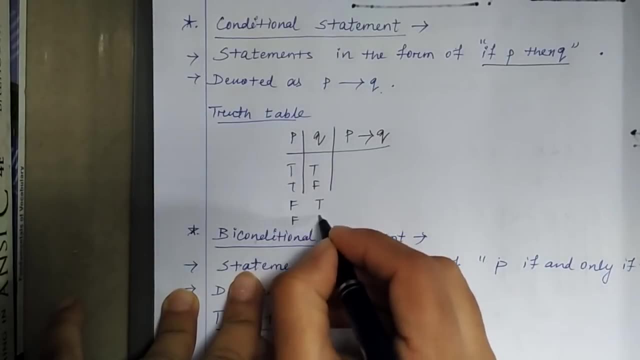 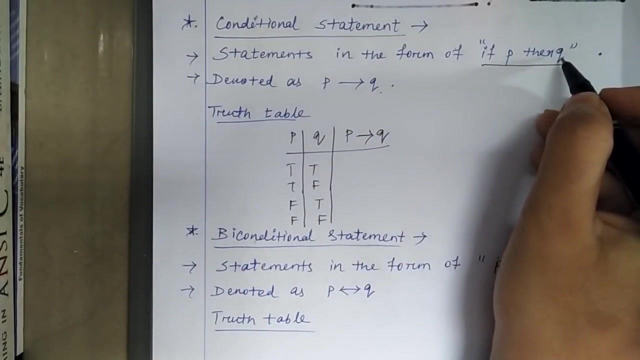 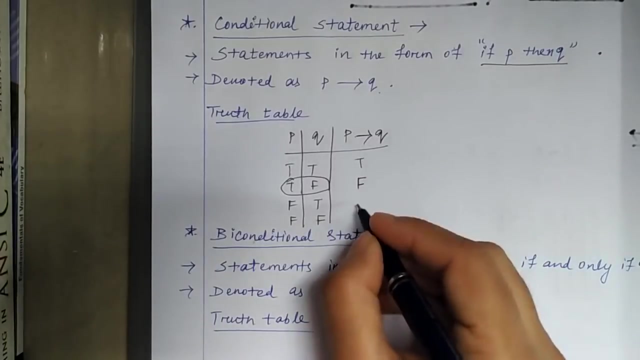 see the truth table of that, that is p, q, p tends to q, and we can write here: p, q is equal to p to q. so true, true, true, false, false, true and false false. if it is if q and then if p and then q is there, then only true false will be false, otherwise rest, all are true. okay, then biconditional. so 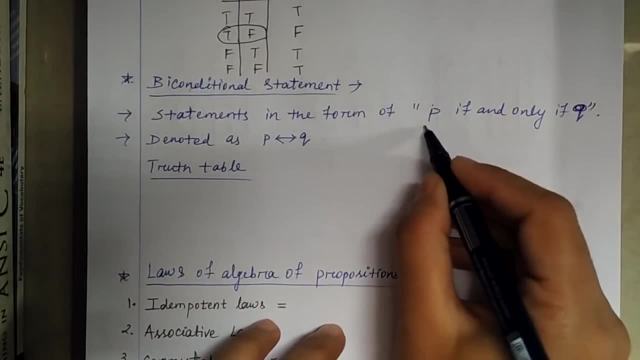 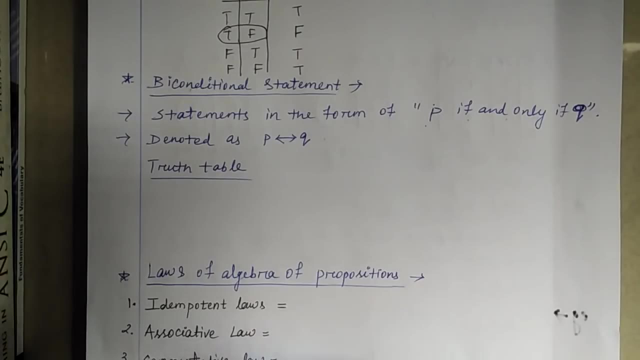 biconditional is if. in the sentence it is of the form p if and only if q. that is in conditional if p, then q in biconditional p if and only if q. so it is denoted as double side arrow symbol. we'll see: